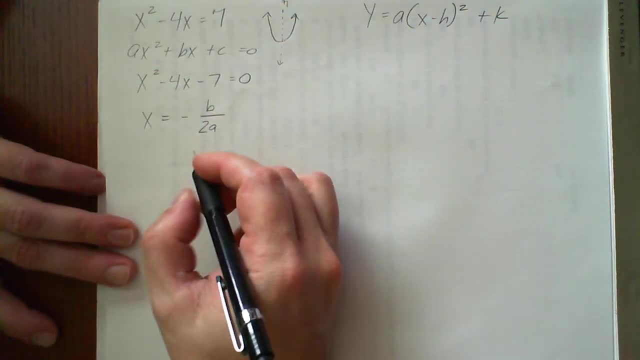 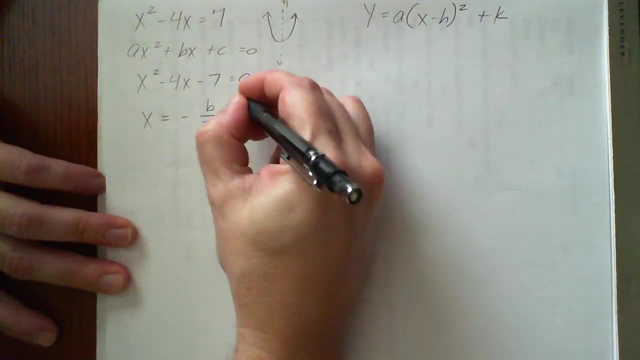 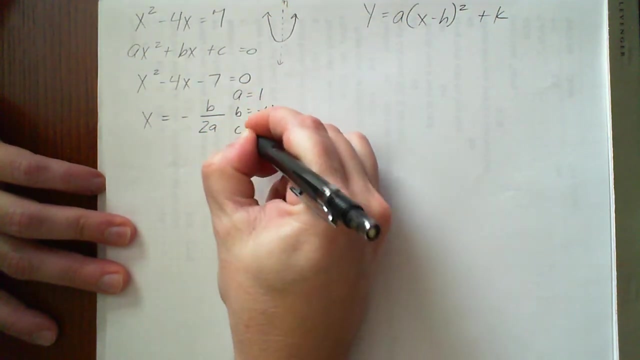 meaning they'll be. x equals some numerical value. Now all I'm going to do is identify. I'm going to identify my a, my b and my c. We don't really need the c value here, but just out of habit, I always write all the values down. 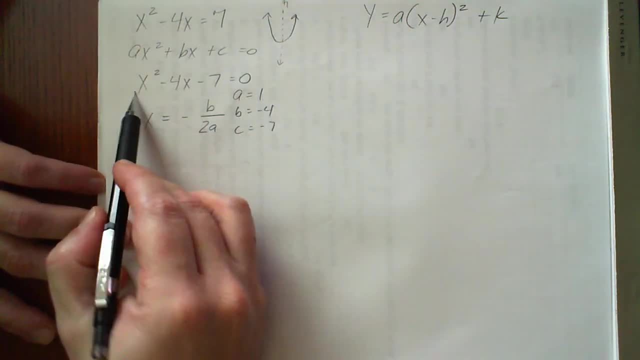 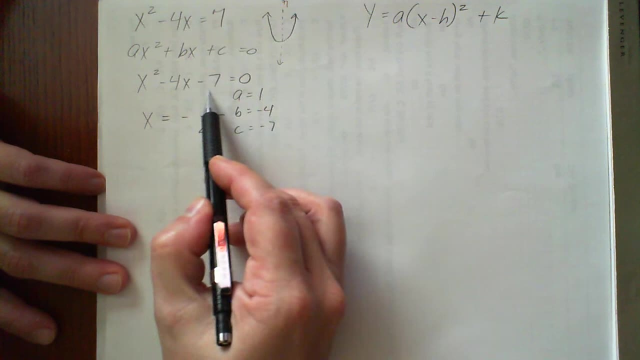 So a is 1, meaning the coefficient of the x squared term, b is negative 4, meaning the coefficient of the x term, And then c is negative 7, which is the constant over here. Like I said, we're not going to use the c value at this point, not for this particular. 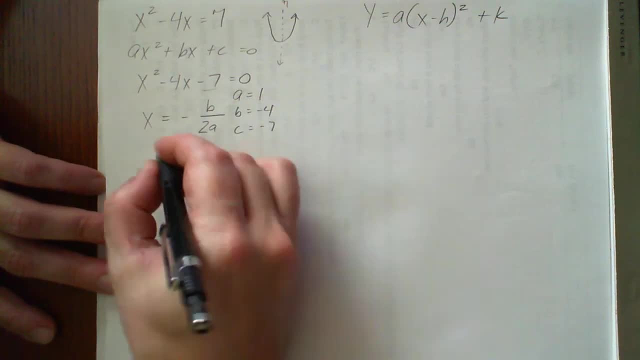 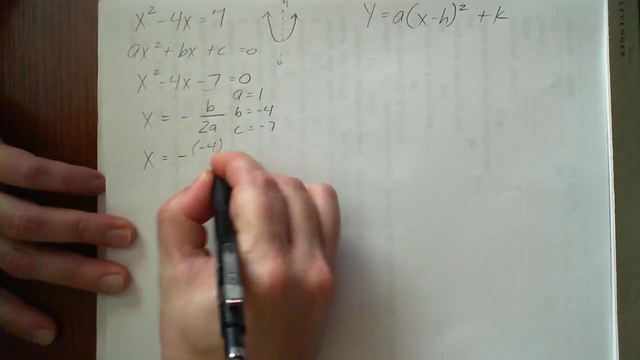 You know purpose of what we're trying to find here, which is just the axis of symmetry. Be careful with your signs here, because my b value is a negative 4.. Remember, you have the existing negative in the formula there, So we do have a negative negative. 4 over 2a is 1, so 2 times 1.. 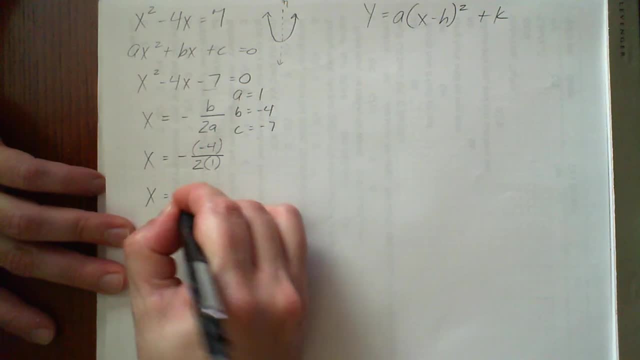 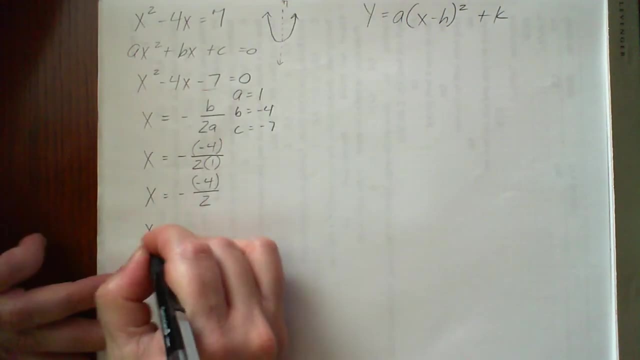 All right, And then continuing, Continuing 2 times 1.. 1 is 2.. Negative 4 divided by 2 is negative 2.. But you have a negative negative 2, which means the opposite of negative 2.. 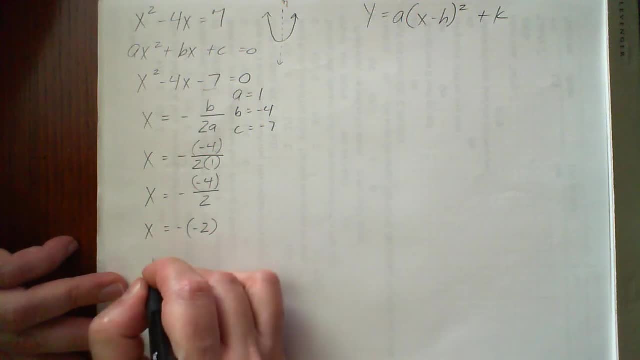 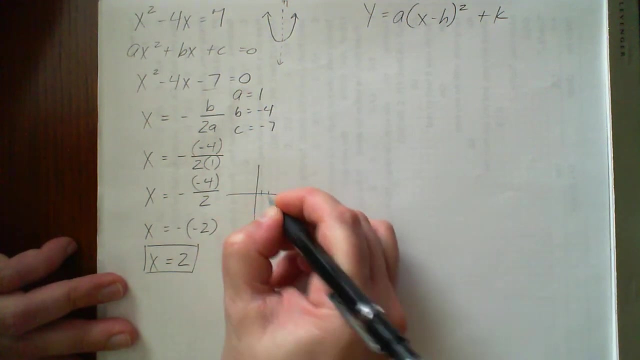 Or you could consider it a negative, 1 times negative, 2.. Either way, it's x equals 2.. That's our axis of symmetry. So when we're thinking of it on a coordinate plane, if I have my x, If I have my y axis, here, here's an x value of 2.. 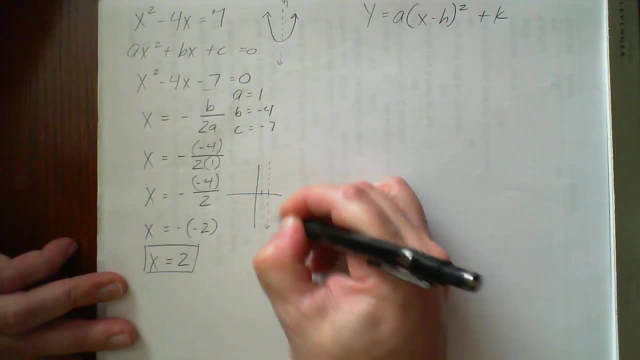 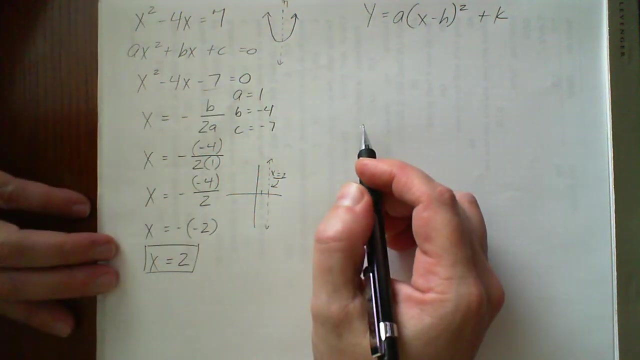 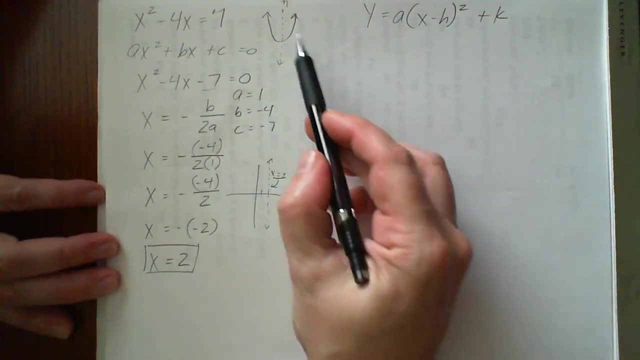 x equals 2 is just a line going through that point 2 on the x axis. All right, Now sometimes we're asked not only to find the axis of symmetry but to find the vertex. Now, when we find a vertex, we're talking about, if we're looking at this parabola, 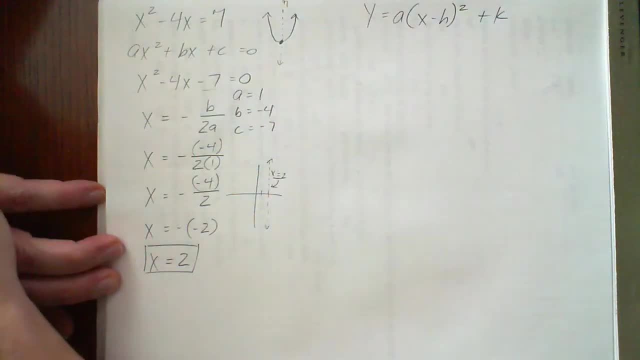 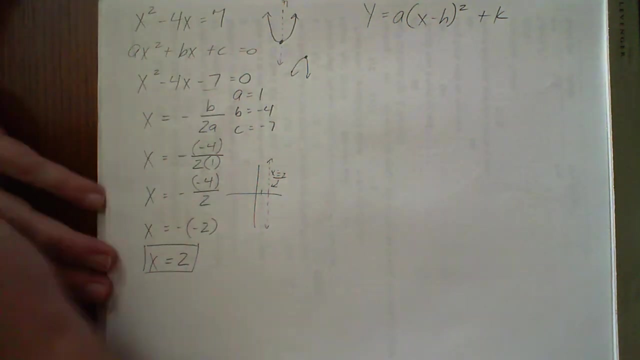 the vertex is this Point right in the center. So you have a parabola sometimes pointing up, sometimes pointing down. The vertex is just right there. You might remember vertex as part of the vocabulary from your geometry course as well. A vertex in that case, you know, we might say the vertex of an angle. 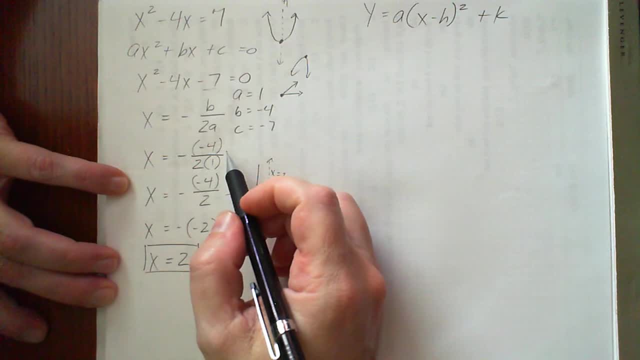 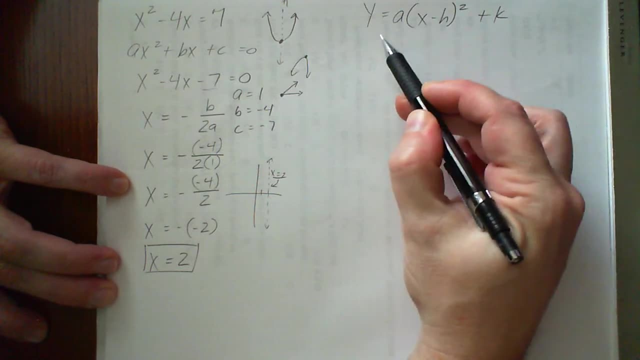 It's just that point here. Or we might say the end of the v or in this case, the end of the u. So we need general form. General form is written here: y equals a times the quantity x minus h squared plus k. 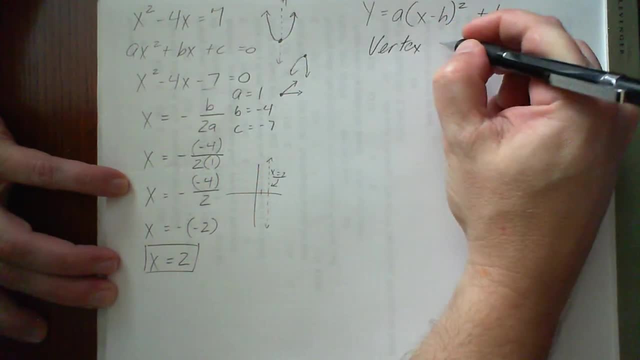 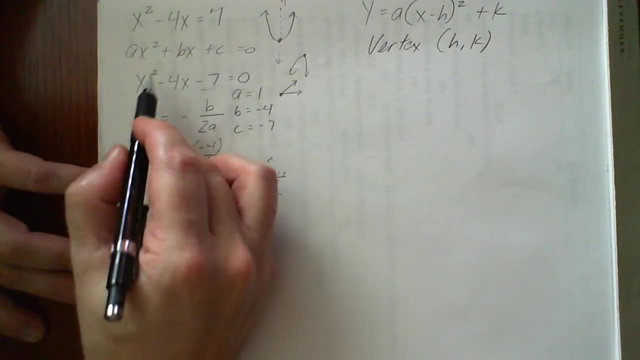 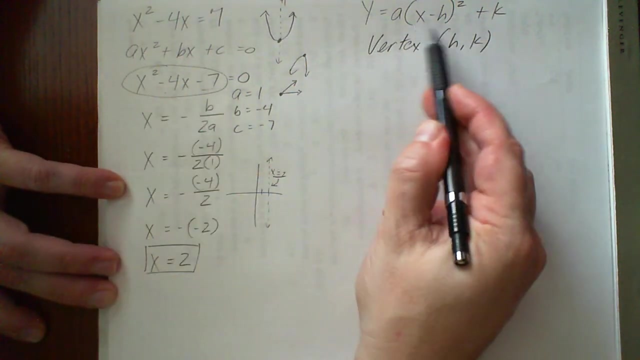 This is a little easier to find our vertex, because the vertex is just h comma k. Now if we look at our- and I'm going to use this, since we've already got the standard form- If we look at this well, we can't really find an h and a k value here. 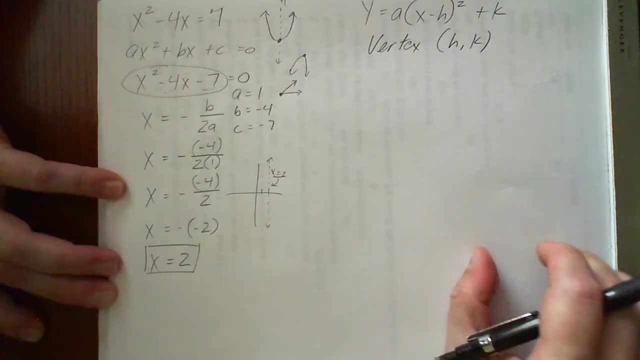 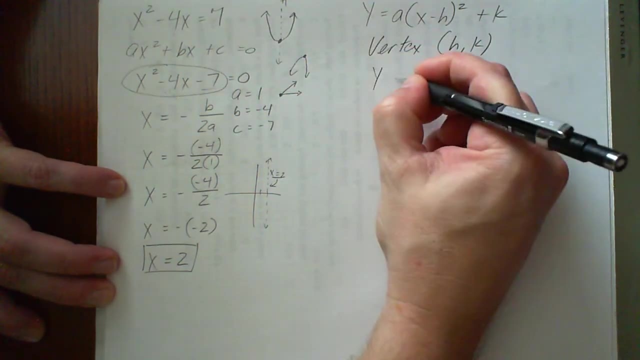 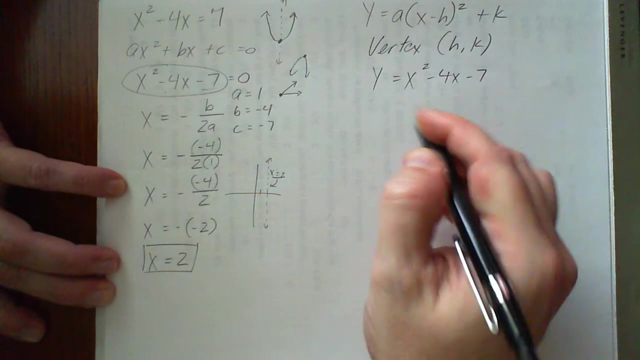 At all. So what we're going to have to do is called: complete the square. When we complete the square, we'll be able to put this into general form. So if y equals x squared minus 4x minus 7, what you'll have to do first is replace your y with 0.. 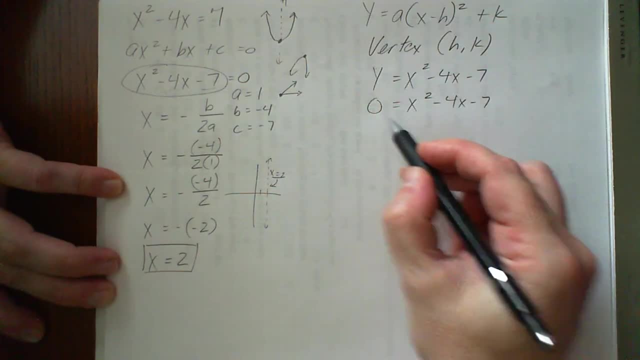 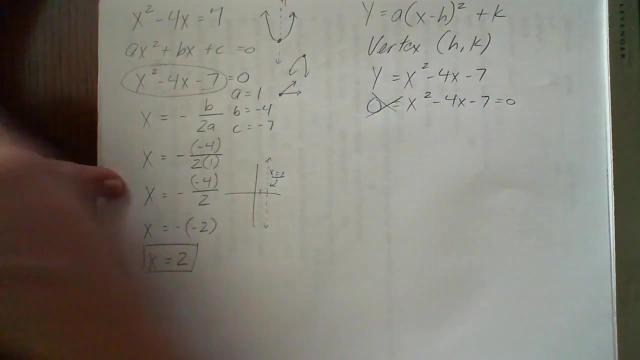 Alright, I really would prefer my 0 to be on the right. I really would prefer my 0 to be on the right. I really would prefer my 0 to be on the right. I'm just going to cross that out and move the equal to 0 over to the right. 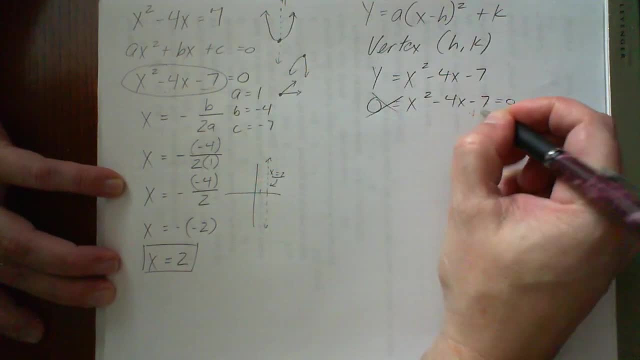 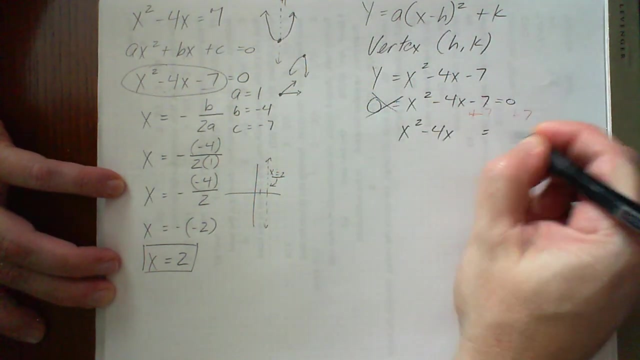 What we're going to do here first is get rid of this 7.. We'll do that by simply adding a 7 to each side. When I add 7 to each side, I'm left with x squared minus 4x equals 0 plus 7, which is 7.. 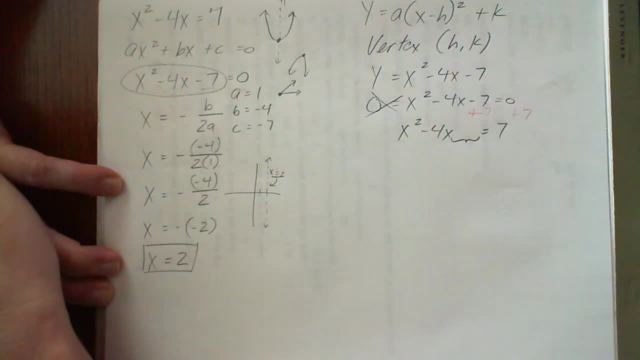 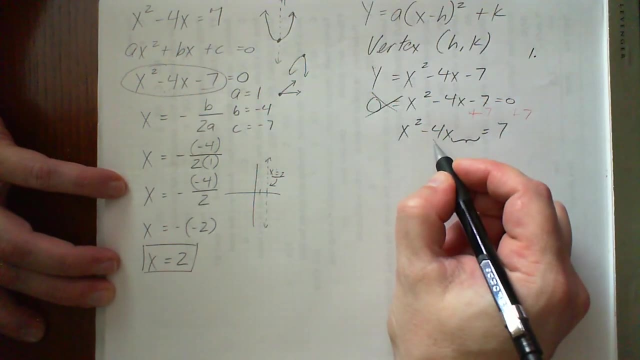 And you'll notice I left a little space right here. So we have specific. So we have specific steps. we're going to do One: I'm going to take the coefficient of my x term and I'm going to cut it in half. 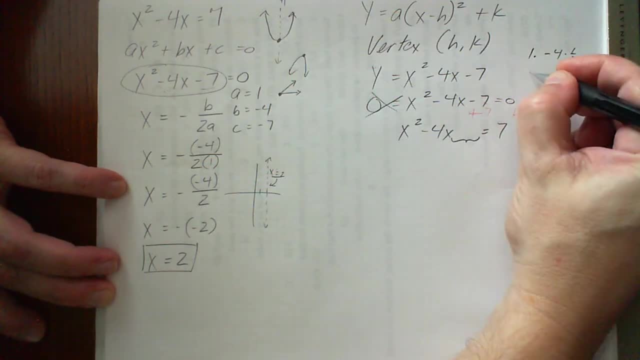 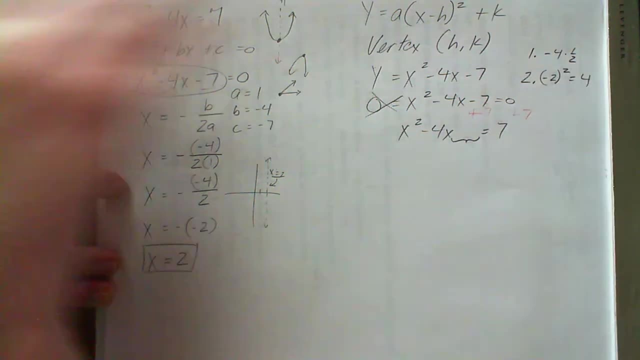 So negative 4 times 1 half, Well, that equals negative 2.. So my next step here is to take that negative 2 and square it. Well, that equals 4.. Now I'm going to use this 4. I'm going to add it to each side of the equation. 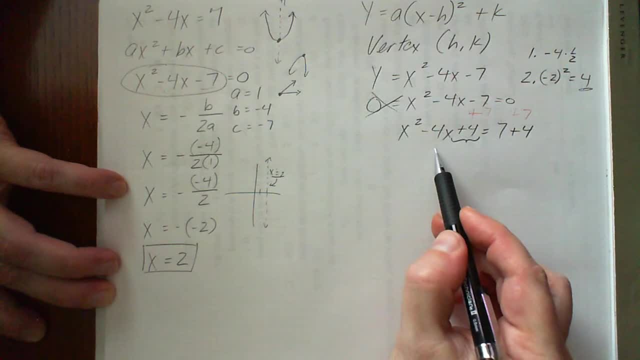 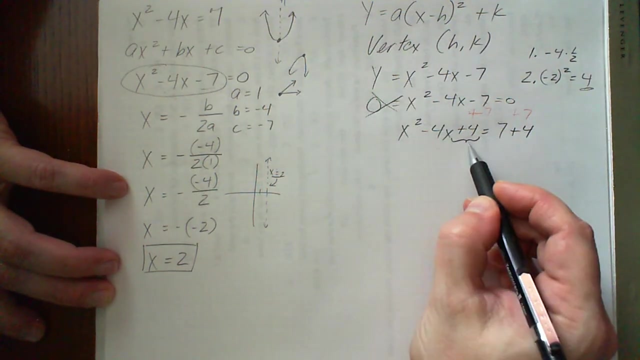 And remember, I can't add something to one side of the equal sign unless I I also add it to the other side of the equal sign. I have to keep everything equivalent as I'm moving through this process. The reason we complete the square is we're creating a perfect square trinomial over here. 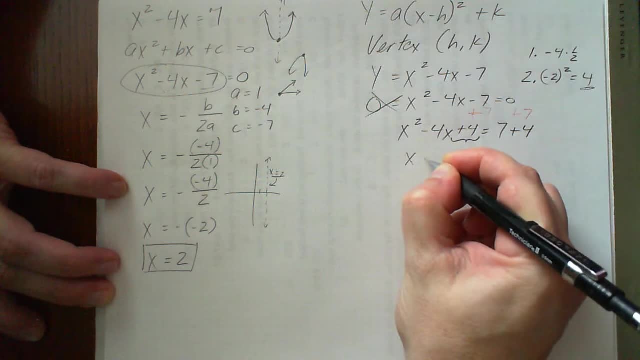 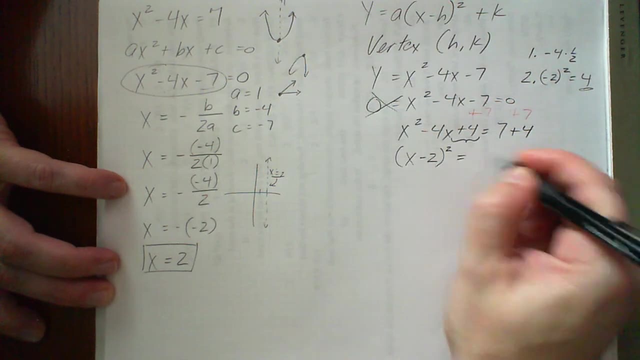 on the left-hand side. So we're going to factor that That's just x minus 2 times x minus 2.. I'm going to write that, as x minus 2 squared equals 7 plus 4 is 11.. Now this still doesn't look exactly. 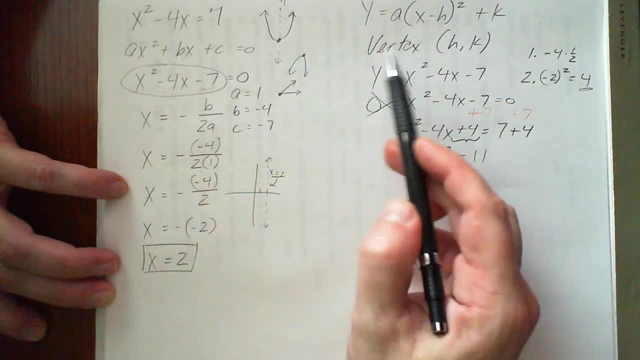 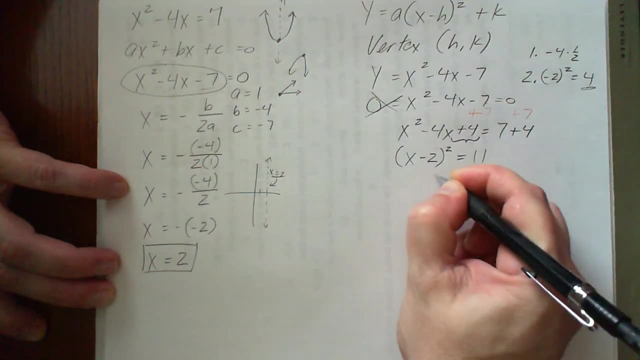 like my general form up here. I need to say y equals and then have something not. This doesn't quite look like that, So we do need to get this 11 back over here. We can do that by subtracting the 11.. 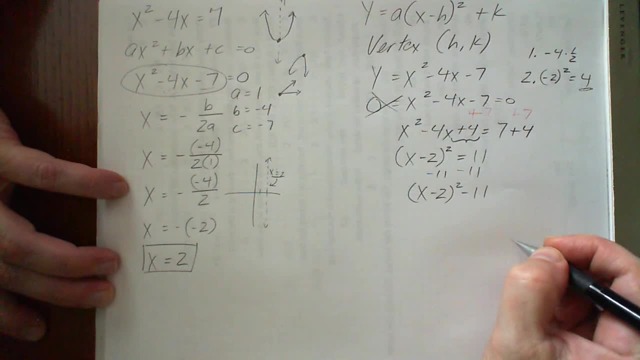 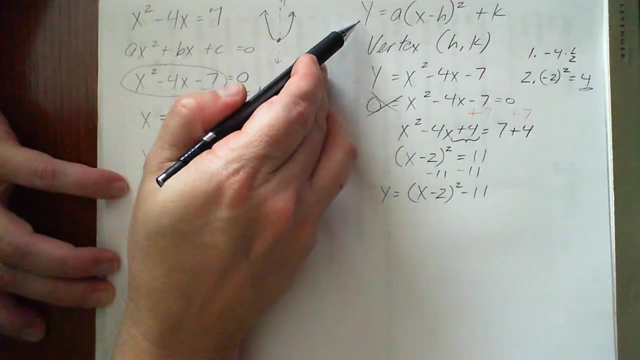 That's going to leave us with x minus 2, squared minus 11.. I could say equal to 0 or 0 equals, but in this case I want it to say y equals, just so it'll be exactly like my general form here. 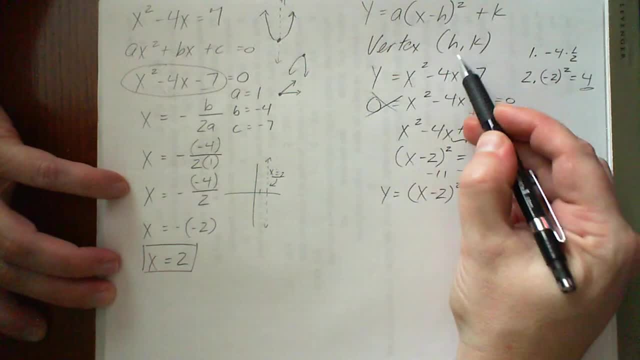 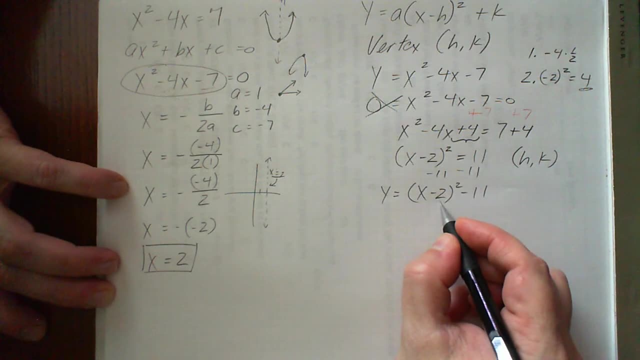 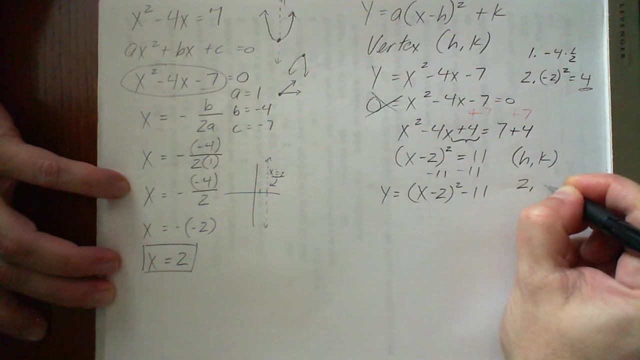 Now remember: our vertex is h comma k, h comma k. Well, in this case our h value- you could see here- is 2.. And our k value is negative 11.. So our vertex here is: 2 comma, negative 11.. 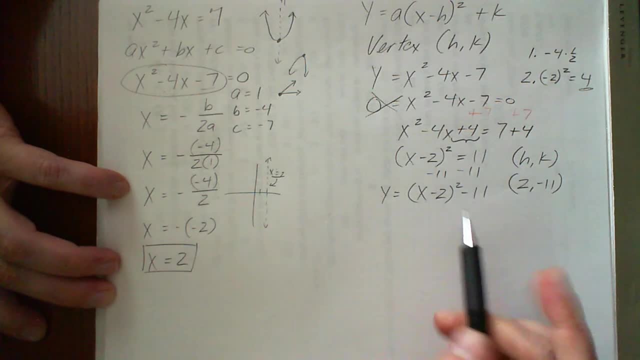 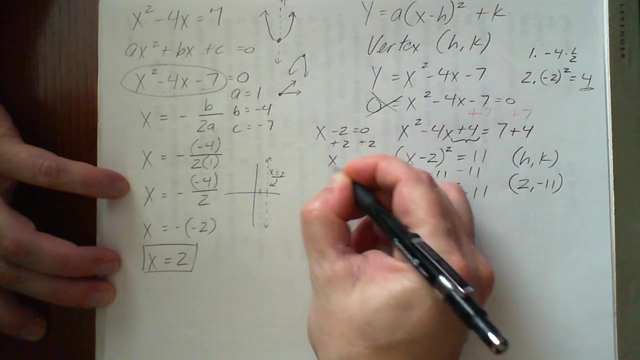 Now we can find the equation of the axis of symmetry, when an equation's in general form, simply by taking this binomial in the parentheses and setting it equal to zero and solving for x. So x minus two equals zero. add two to each side and x equals two. You'll notice that obviously we end up with the. 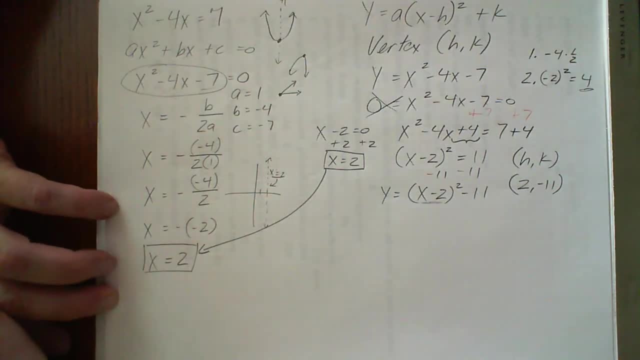 same answer, regardless of the method we use to find that value. Now that I know my axis of symmetry and my vertex, you also notice that the axis of symmetry, which is an equation, it's a linear equation. x equals some value. It's a vertical line, but it's always going to be the x value of. 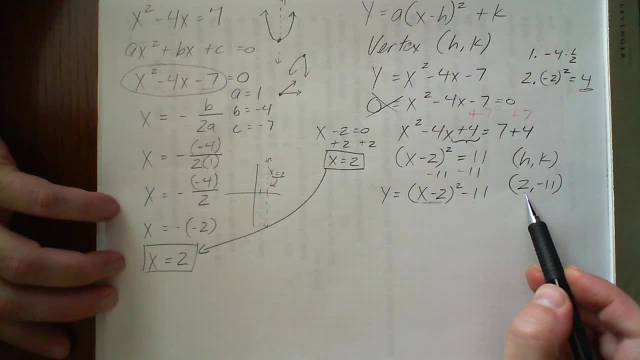 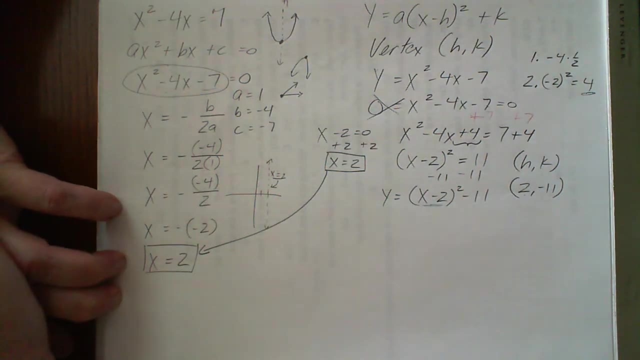 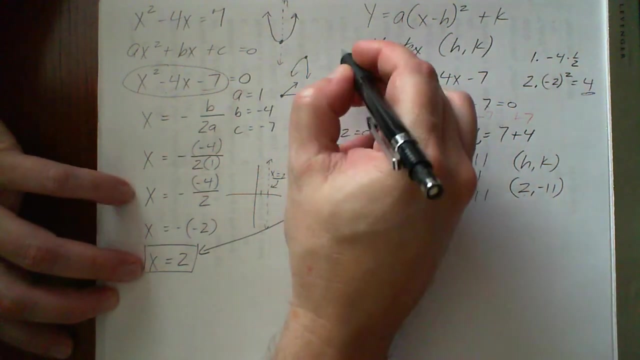 your vertex. So it's another way to think of what is my axis of symmetry? Well, it's just the x value of the vertex. So we have several ways we can determine the axis of symmetry. Since I have the axis of symmetry and the vertex, you could make a quick sketch of that graph. It would look: